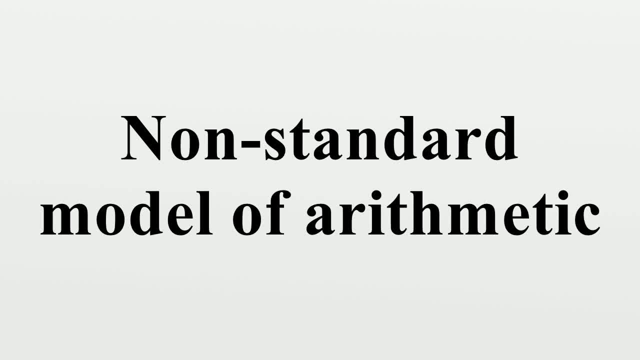 In mathematical logic. a non-standard model of arithmetic is a model of Pinot arithmetic that contains non-standard numbers. The term standard model of arithmetic refers to the standard natural numbers, chapter 0,, 1, 2.. The elements of any model of Pinot arithmetic are linearly ordered and possess an initial segment isomorphic to the standard natural numbers. 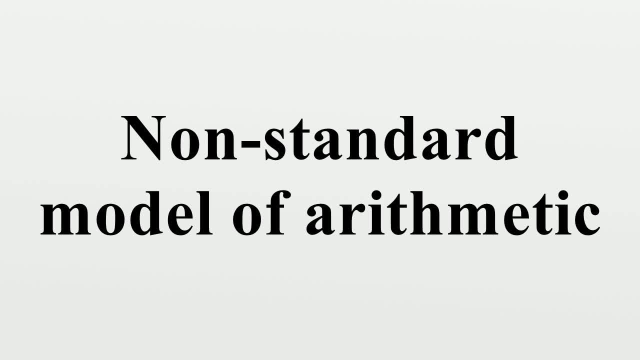 A non-standard model is one that has additional elements outside this initial segment. The construction of such models is due to Thor-Alf Skolum existence. There are several methods that can be used to prove the existence of non-standard models of arithmetic From the compactness theorem. the existence of non-standard models of arithmetic can be demonstrated by an application of the compactness theorem. 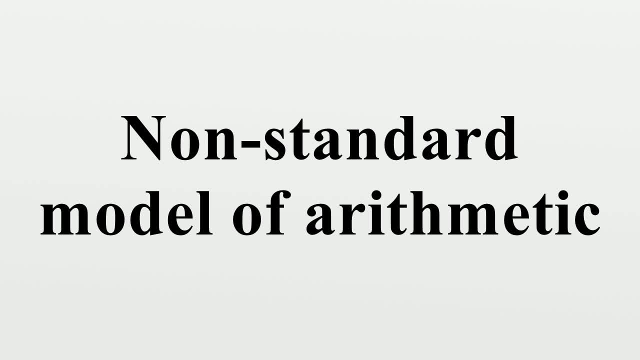 To do this, a set of axioms- P, asterisk- Asterisk- is defined in a language including the language of Pinot arithmetic, together with a new constant symbol, x. The axioms consist of the axioms of Pinot arithmetic P, together with another infinite set of axioms for each numeral n. 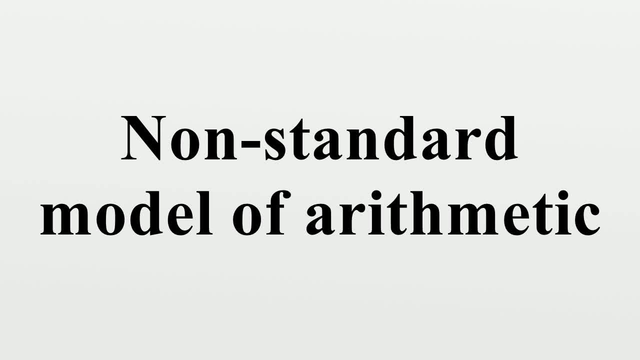 The axiom x greater than n is included. Any finite subset of these axioms is satisfied by a model that is the standard model of arithmetic, plus the constant x, interpreted as some number Larger than any numeral Mentioned in the finite subset of P asterisk. 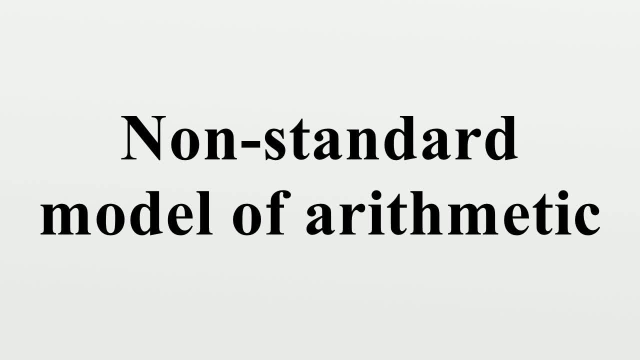 Thus, by the compactness theorem, there is a model satisfying all the axioms: P asterisk. Since any model of P asterisk is a model of P, we have that our extended model is also a model of the Pinot axioms. The element of this model corresponding to x cannot be a standard number because, as indicated, it is larger than any standard number. 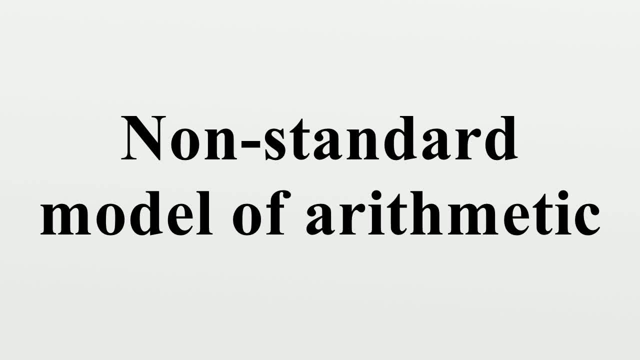 Using more complex methods It is possible to Build non-standard models that possess more complicated properties. For example, there are models of Pinot arithmetic in which Goodstein's theorem fails. It can be proved in Zamello-Frankel set theory that Goodstein's theorem holds in the standard model. 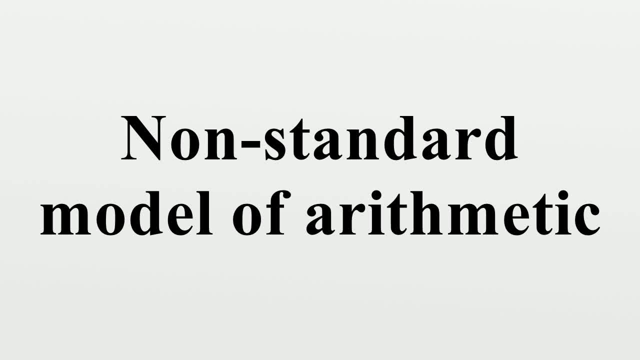 So a model where Goodstein's theorem fails must be non-standard From the incompleteness theorems. Godel's incompleteness theorems also imply the existence of non-standard models of arithmetic. The incompleteness theorems show that a particular sentence g 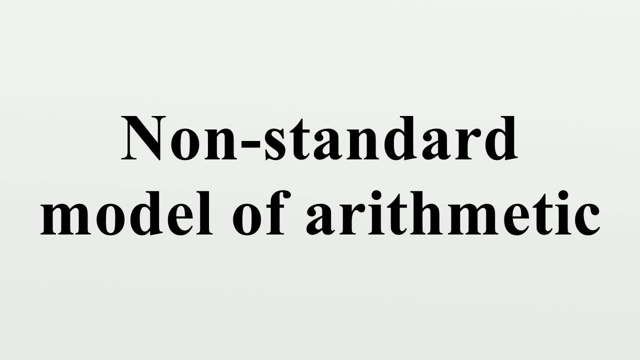 The Godel sentence of Pinot arithmetic is not provable, nor disprovable in Pinot arithmetic By the completeness theorem. this means that g is false in some model of Pinot arithmetic. However, g is true in the standard model of arithmetic And therefore any model in which g is false must be a non-standard model. 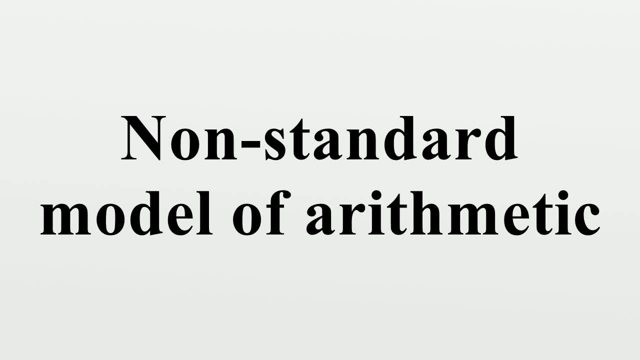 Thus satisfying tilde g is a sufficient condition For a model to be non-standard. it is not a necessary condition, However, for any Godel sentence g. there are models of arithmetic with g true of all cardinalities. Arithmetic unsoundness for models with tilde g: true, assuming that arithmetic is consistent. 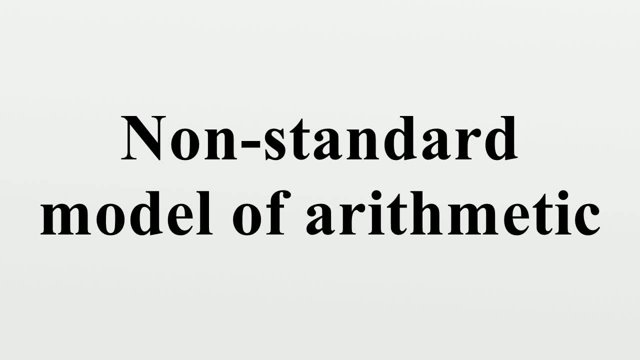 Arithmetic with tilde g is also consistent. However, since tilde g means that arithmetic is inconsistent, The result will not be omega consistent From an ultraproduct. another method for constructing a non-standard model of arithmetic is via an ultraproduct. 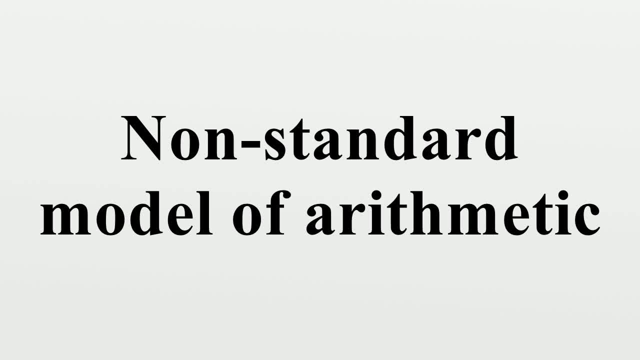 A typical construction uses the set of all sequences of natural numbers. Identify two sequences if they agree for a set of indices that is a member of a fixed, non-principle ultrafilter. The resulting semi-ring is a non-standard model of arithmetic. It can be identified with the hypernatural numbers. 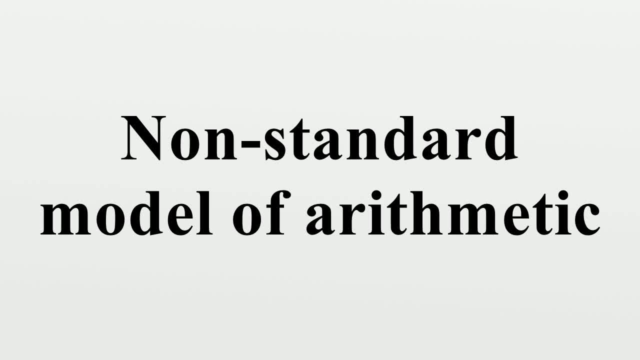 Structure of countable numbers. Countable non-standard models. The ultraproduct models, are uncountable. One way to see this is to construct an injection of the infinite products of n into the ultraproduct. However, by the Loewenheim-Scolum theorem, there must exist countable non-standard models of arithmetic. 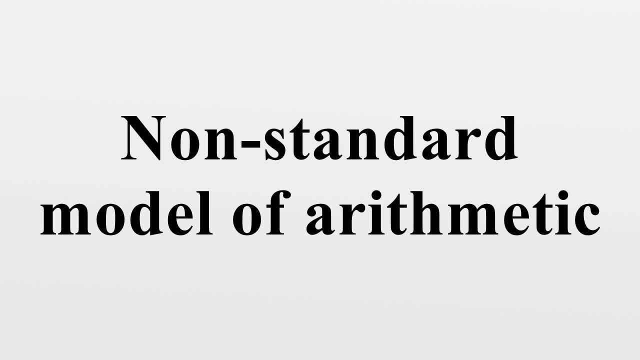 One way to define such a model is to use Henck and semantics. Any countable non-standard model of arithmetic has order type omega plus eta, Where omega is the order The type of the standard natural numbers, Omega asterisk is the dual order and eta is the order type of the rational numbers. 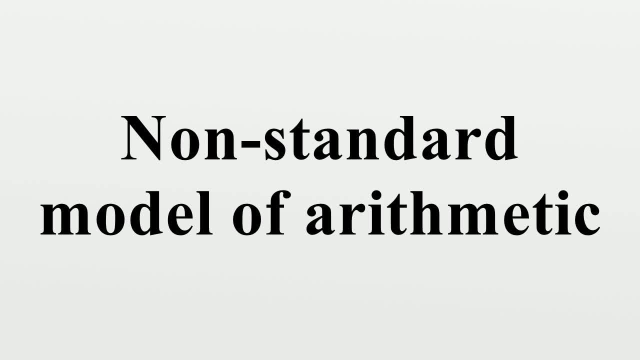 In other words, a countable non-standard model begins with an infinite increasing sequence. This is followed by a collection of blocks, each of order type omega, asterisk, plus omega, the order type of the integers. These blocks are, in turn, densely ordered with the order type of the rationals. 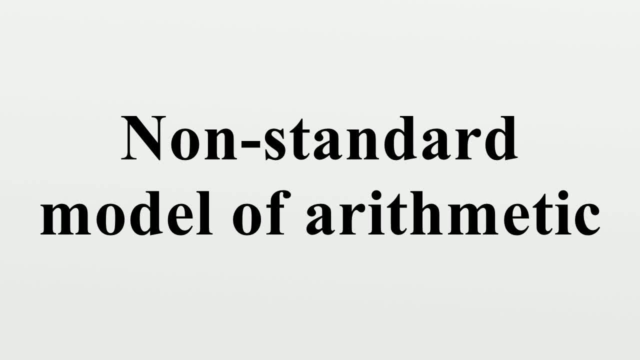 The result follows fairly easily because it is iterative. It is easy to see that the non-standard numbers have to be dense and linearly ordered without endpoints And the order type of the rationals is the only countable dense, linear order without endpoints. So the order type of the countable non-standard models is known. 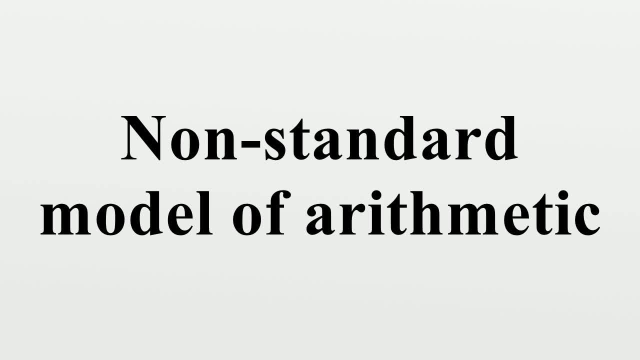 However, the arithmetical operations are much more complicated. It is easy to see that the arithmetical structure differs from omega plus eta, For instance, if u is in the model, then so is m asterisk u for any m n in the initial segment n. yet u2 is larger than m asterisk u for any standard finite m. 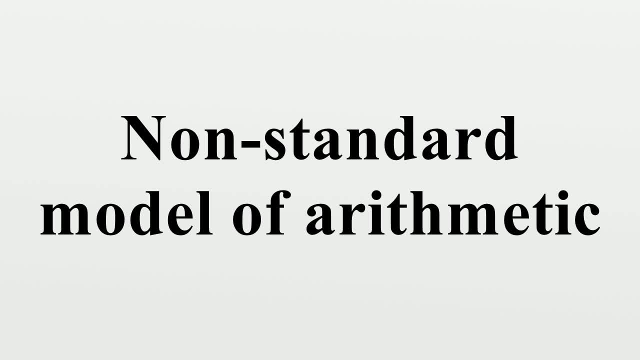 Also, you can define square roots such as the least v, such that v2 greater than 2 asterisk u. It is easy to see that these can't be within a standard finite number of any rational multiple of u. By analogous methods to non-standard analysis, you can also use PAR to define close approximations to a rational multiple. 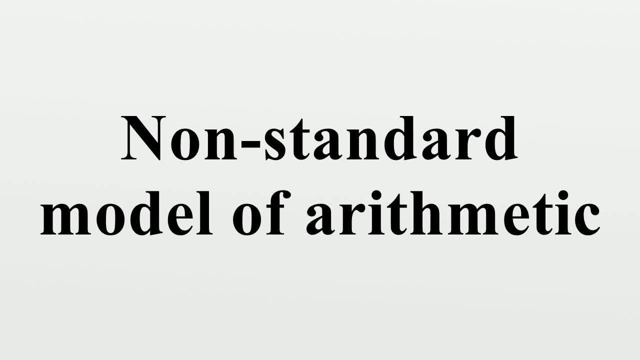 For example, if u is in the model, then so is m asterisk u for any m n in the initial segment, n yet u2 greater than 2 asterisk u. Also, you can define square roots such as the least v, such that v2 greater than 2 asterisk u. 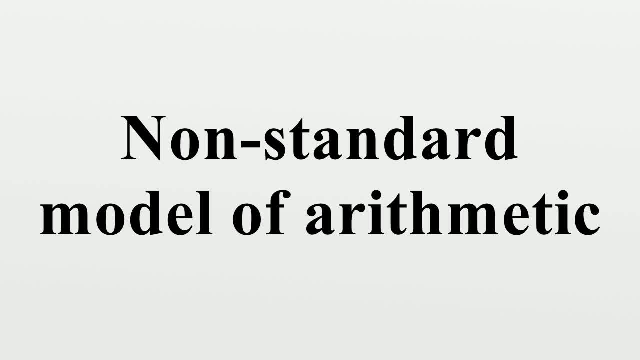 Once more, v asterisk u n has to be larger than any standard finite number for any standard finite m n. This shows that the arithmetical structure of a countable non-standard model is more complex than the structure of the rationals. 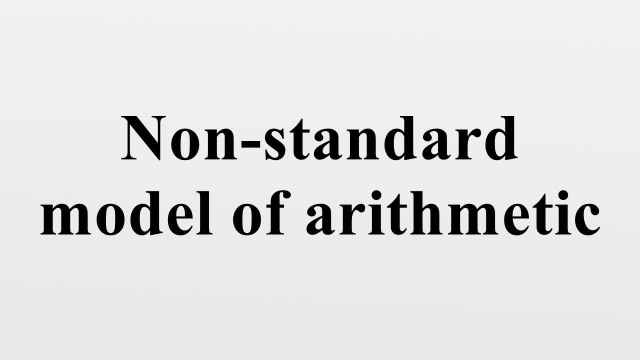 There is more to it than that, though. Tenant-Boum's theorem shows that for any countable non-standard model of p, there is no way to code the elements of the model as natural numbers, such that either the addition or multiplication operation of the model is a computable on the codes. 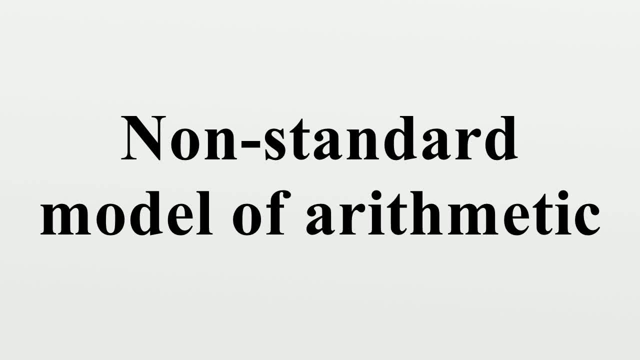 This result was first obtained by Stanley Tenant-Boum in 1959.. Citations: Carrot-André Bovikin and Richard B K. Order: types of models of Pino. arithmetic- A short survey, June 14, 2001. 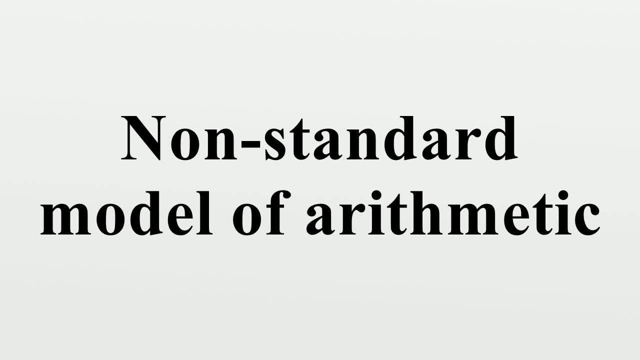 Carrot-André Bovikin on order: types of models of arithmetic. thesis submitted to the University of Birmingham for the degree of PhD in the Faculty of Science, 13 April 2000. Carrot-Linear orders: Discrete, dense and continuous. 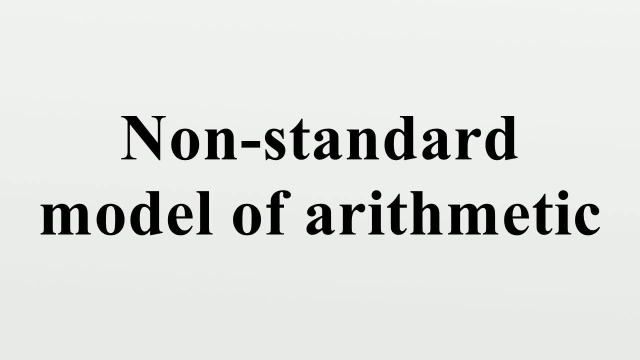 includes proof that q is the only countable dense linear order. 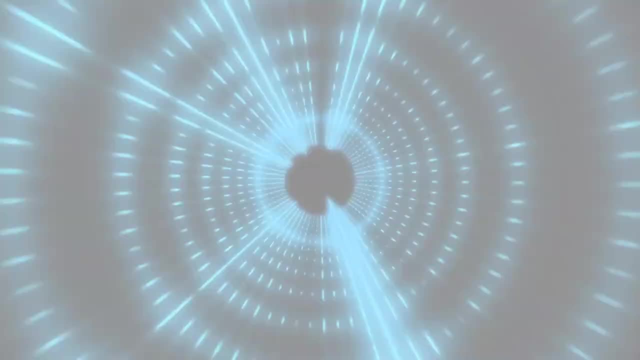 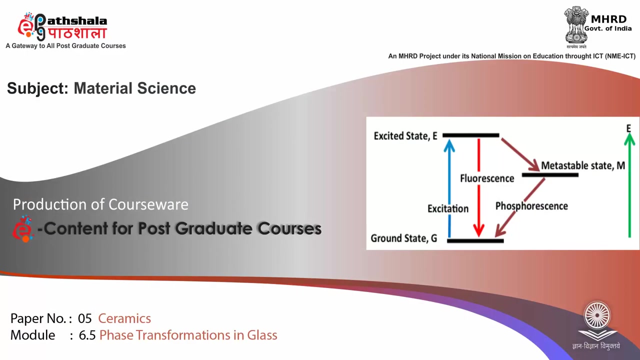 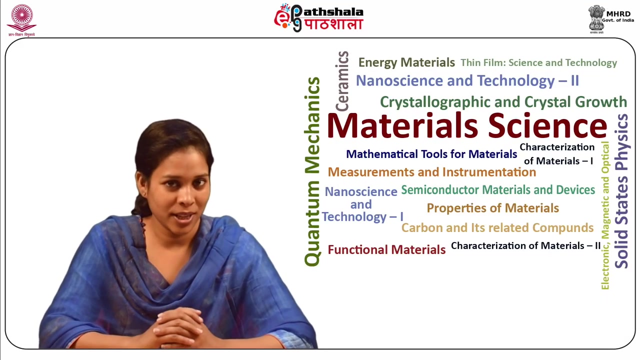 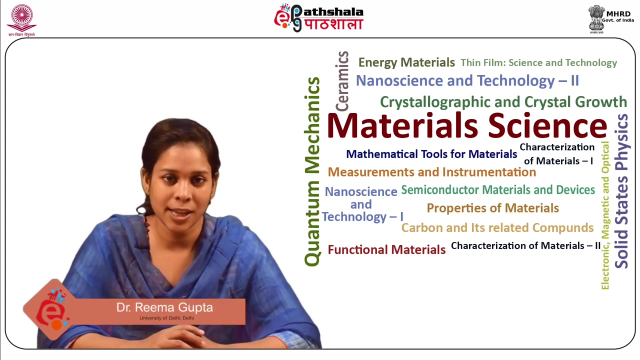 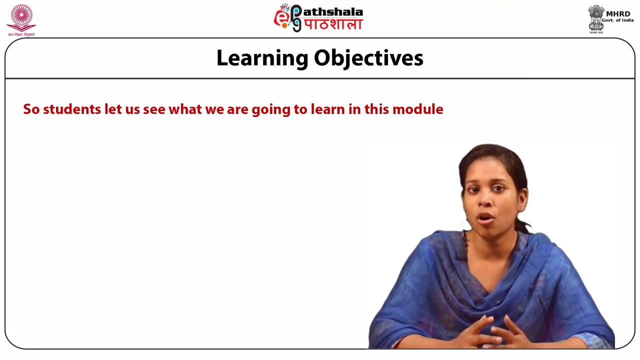 Hello students, welcome to EPG Parchala. I am Rima Gupta from University of Delhi and today we are going to talk on module Structural Theory of Glass Formation, and this module is under the paper Ceramics. So, students, after the completion of this module, you all should be able: 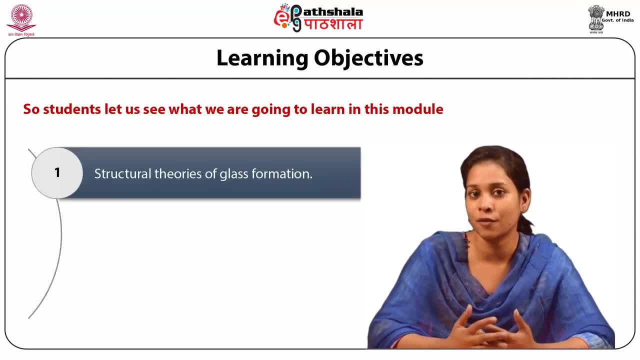 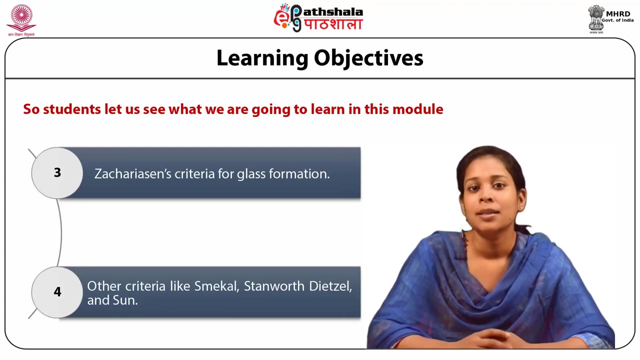 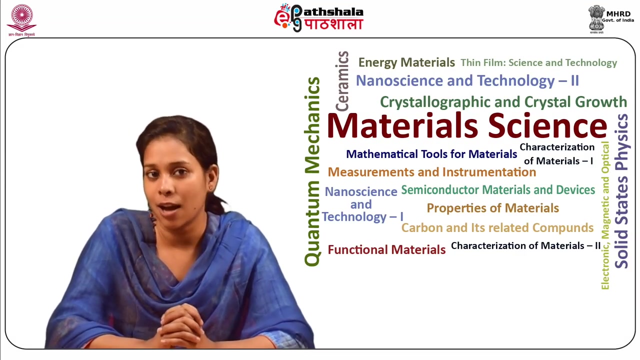 to understand the structural theories of glass formation, which includes Goldsmith's radius ratio criteria, the Shearishan criteria for glass formation and various other criteria like Schmeichel, Stanford, Ditzel and Sun. So here comes phase transformations in glass. A glass can. 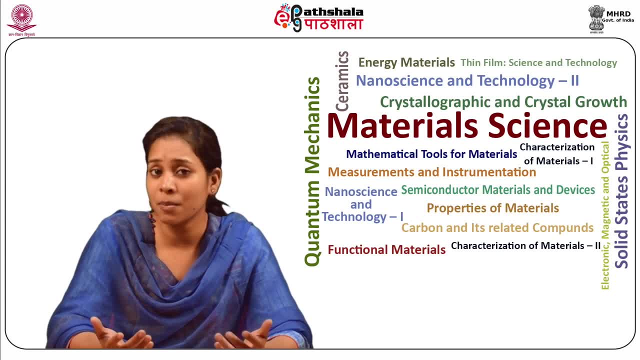 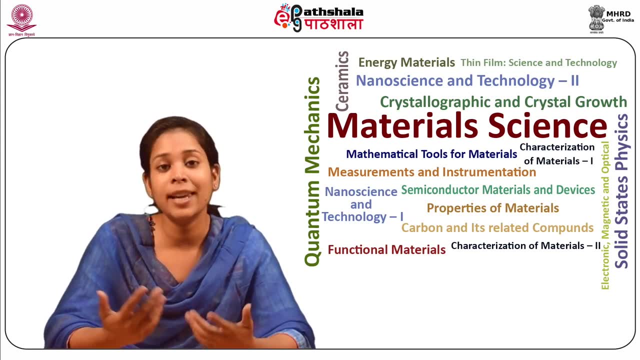 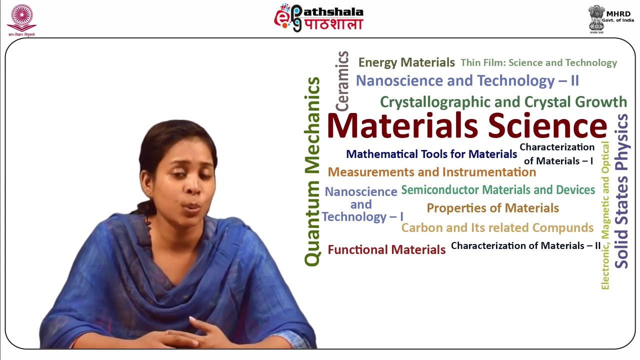 undergo several types of phase transformations. It can crystallize into a crystalline phase or it can undergo liquid phase separation. These two types of phase transformation can occur in more than one way. These are shown already in the figure. The crystallization may occur from the liquid phase or if the liquid is cooled to a glass. 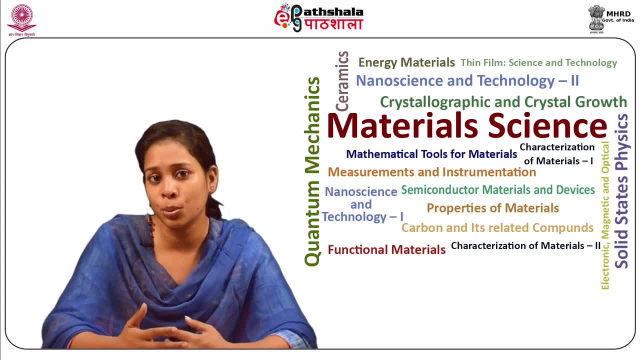 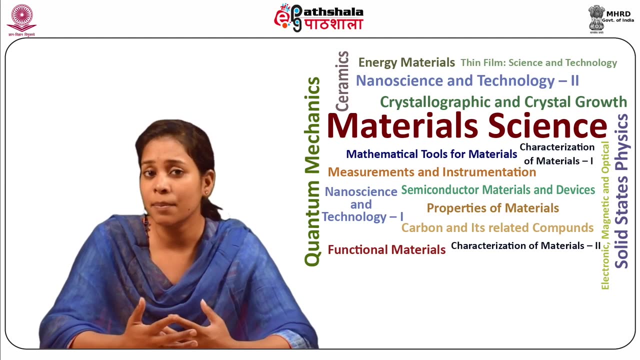 phase, then crystallization may be induced by subsequent heating of the solid glass below the liquid formation temperature, Whereas the later case is the procedure used to produce the glass ceramics, as discussed in later slides. The crystallization occurs by nucleization and growth. It may occur on the surface or in the bulk of the glass. The nucleation- may be homogenous nucleation or in the form of the massive formation process. It can be của chrystallization by nucleization and growth, As encouraged read by P? S work. So channeling of our luck. State- dentistry canal. the Hardware System is known as the capital for Cont? 즐 nhs level surgery.